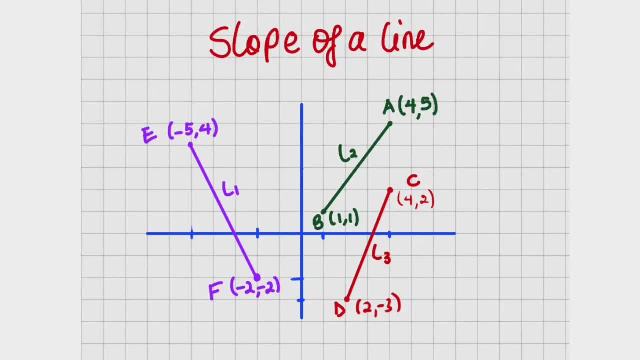 Hello, good day viewers. In this tutorial, I'm going to show you two different ways to find the slope or a gradient of any given line. We have three lines, L1 to L3, and we want to find their corresponding slopes. Okay, let me show you the two different ways. We have the first way, m, which is 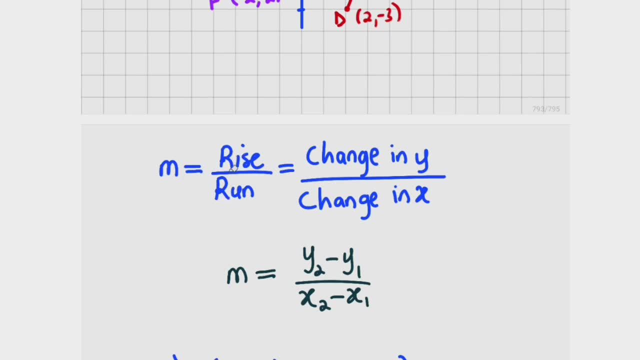 the slope equal to rise divided by the run. Rise stands for the change in y, while the run stands for the change in x. or you can always use the formula m equal to y2 minus y1 divided by x2 minus x1.. So let's start with the first one, which is rise over run. You can always form a right angle. 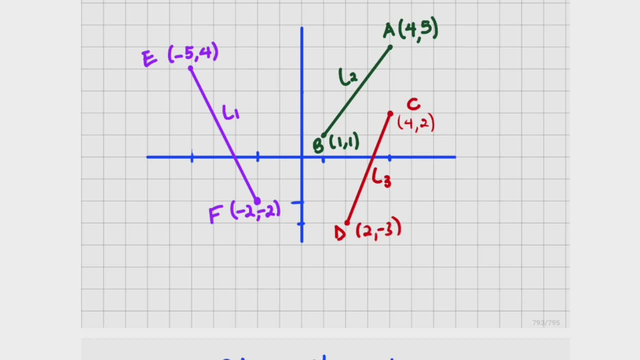 triangle at two given points. You can choose any two given points, but since this is a line segment, we have end to end points. So let's construct a right angle triangle on the line EF. So we have right angle triangle like this Rise. here is the change in y, so you count the changes: one, two, three, four, five, six. 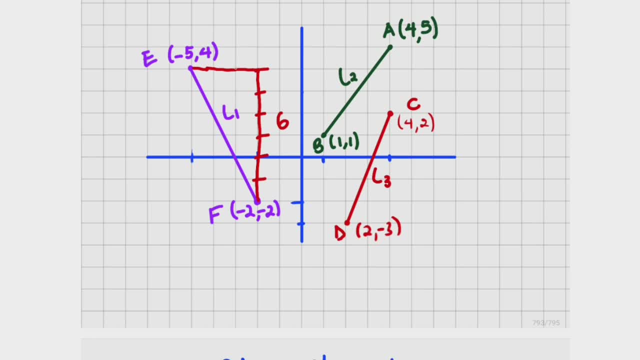 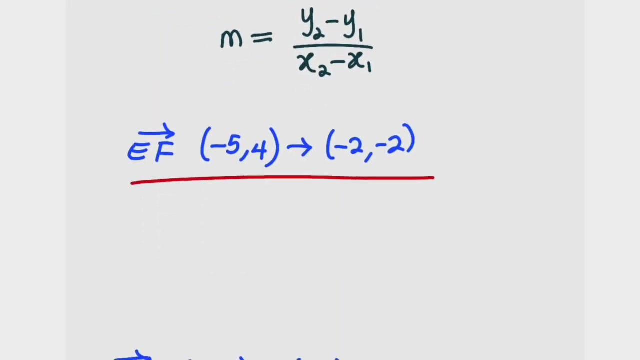 So in change in y, we have six. What about change in x? We have one, two, three. Since we are moving to the left, we have negative three. Therefore, the slope is what Six divided by negative three? Then you write it here. You can see I have already formed the line here. The slope is equal to: 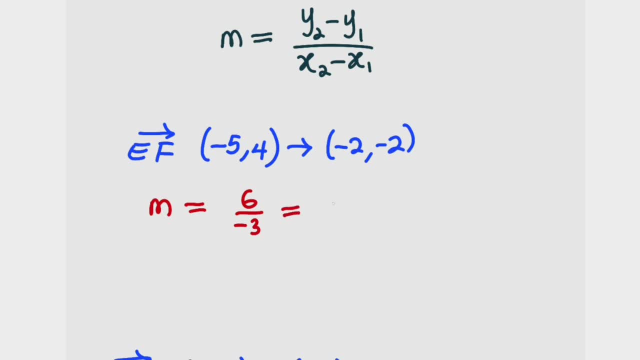 six divided by negative three, which is equal to what Negative two. And you can use the second method, which is y2 minus y1 divided by x2 minus x1.. If this is x1 and this is y1, this should be x2 and this should be y2.. Applying this formula- y2 minus y1 divided by x2 minus x1- we have the slope to be. 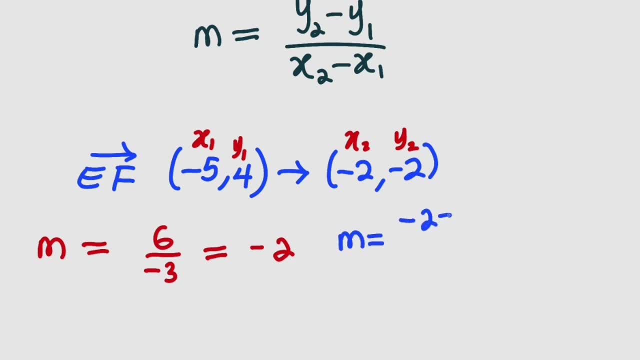 negative three. And if this is x1 and this is y2, we have the slope to be negative two. So now let's say we have the slope here. We have y2 equal to y2, which is negative two minus y1, which is what. 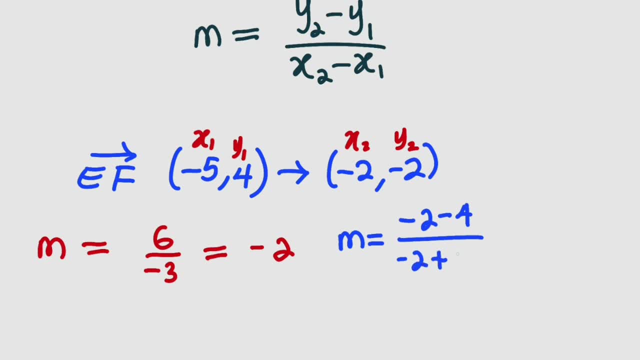 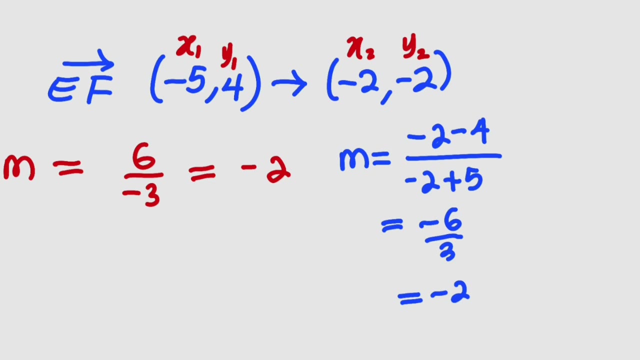 Four divided by x2, which is negative two, minus x1, which is negative five. So this becomes positive five. To the top, we have negative six. To the bottom, we have three, And if you simplify this, you're going to obtain negative two. You see, in each case we have the same answer: negative two. 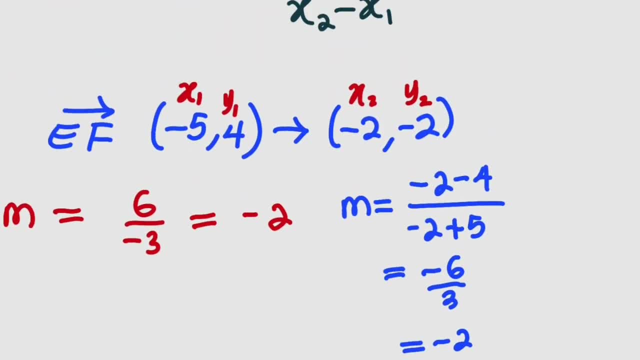 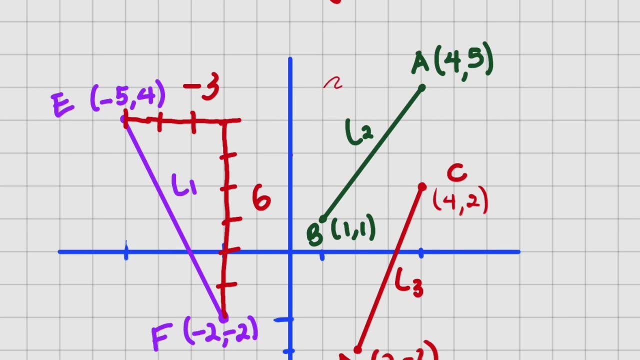 So now let us move on to the second line, which is line AB. You can see line AB here. You can also form a right angle triangle from bottom to the top. So what is the change? in Y, We have 1,, 2,, 3,, 4.. 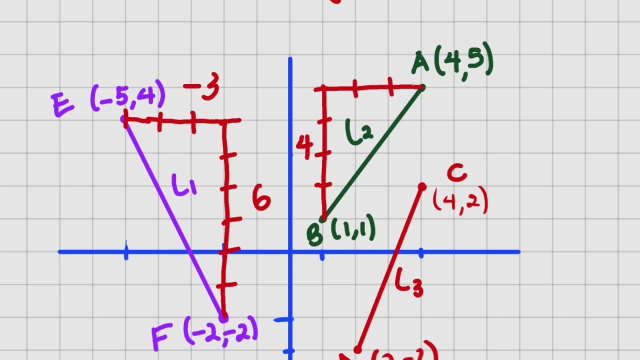 This is 4, right And change in X is 1,, 2, 3.. We are going to consider it as positive 3 because we are moving to the right. So the slope is going to give us 4 divided by 3.. 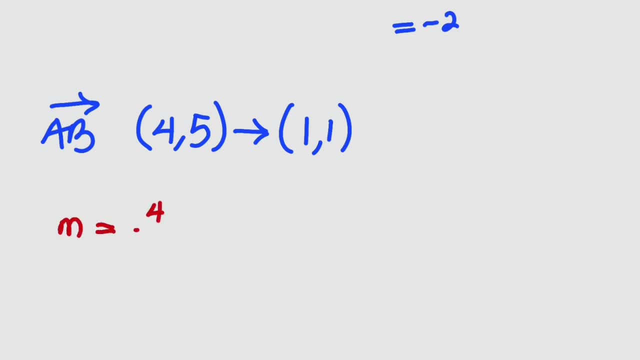 So the slope M is rise over, run. as simple as that. This is the slope. So now let us apply the formula and we can start from any given point. So I can call this one X2.. This is Y2.. This is X1.. 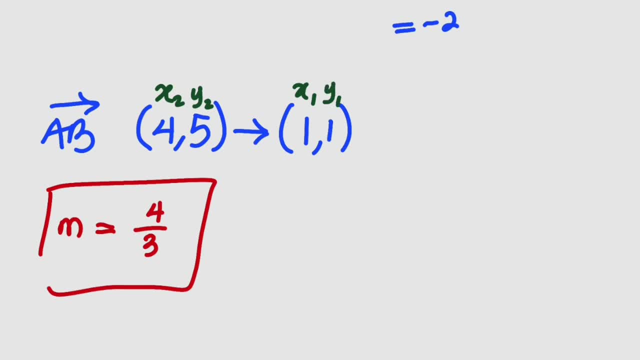 This is Y1.. I told you you can start from any point, So the slope M is equal to Y2, which is 5., Minus Y1, which is 1, divided by X2, which is 4, minus X1, which is 1.. 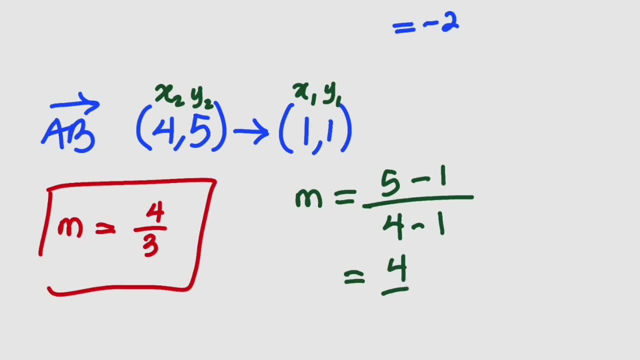 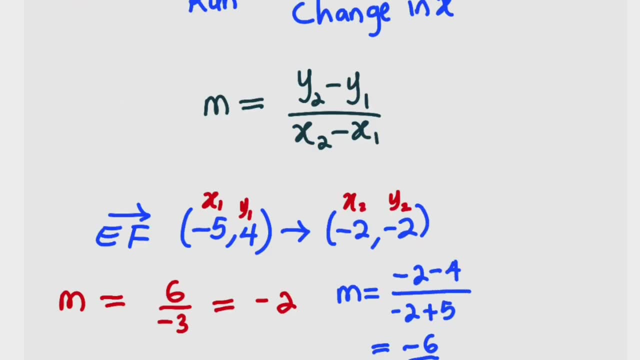 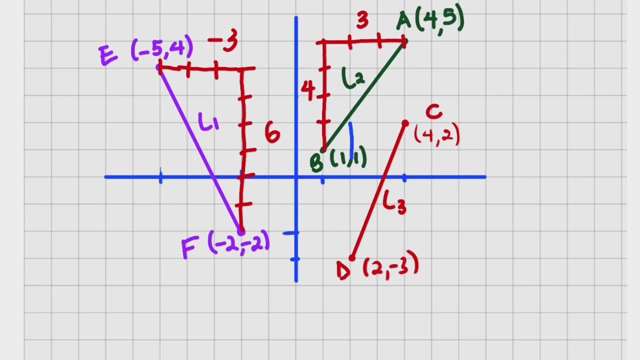 This is equal to 5 minus 1 is 4, and 4 minus 1 is 3.. You can see. they are exactly the same. So let us take the last one, which is line CD, Line CD. Let us form a right angle triangle as well. 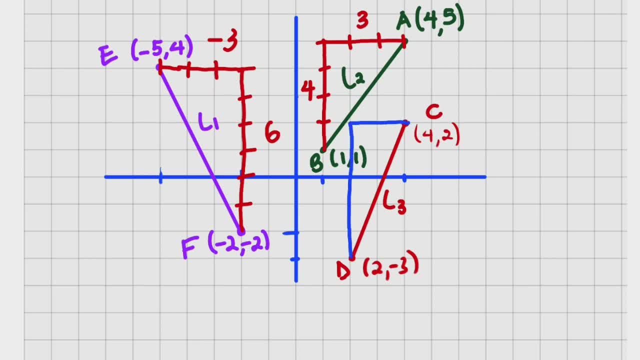 We have this from bottom to the top. What is change in Y? Let us count 1,, 2,, 3,, 4, 5.. So change in Y is 5.. Change in X is 1, 2.. 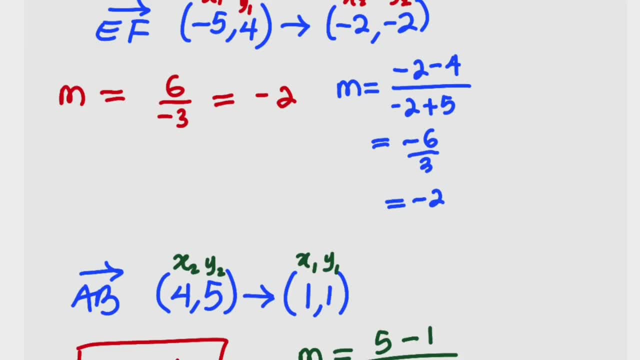 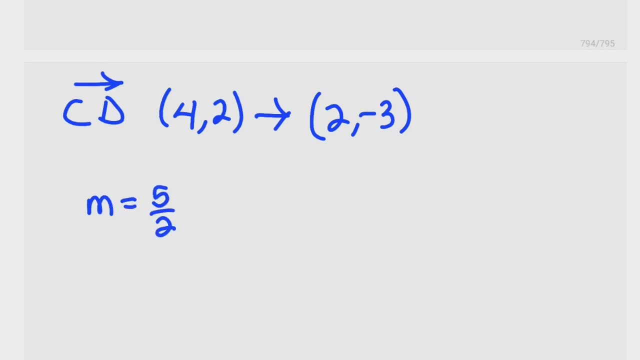 So we have 2 here. Therefore the slope is 5 divided by 2.. So the slope here is equal to 5 divided by 2.. And if we apply the formula Y2 minus Y1 divided by X2 minus X1,, let me call this one as Y2.. 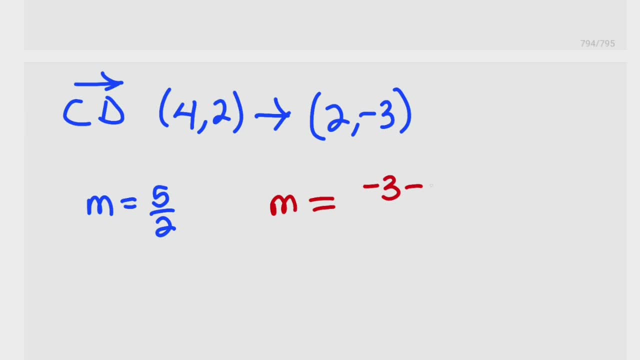 So we have negative 3.. Minus Y1,, which is 2, divided by X2, minus X1,, which is 4.. So this is equal to to the top. we have negative 3, negative 2 is negative 5..